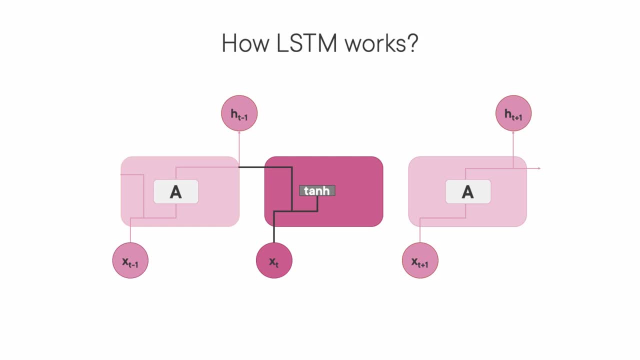 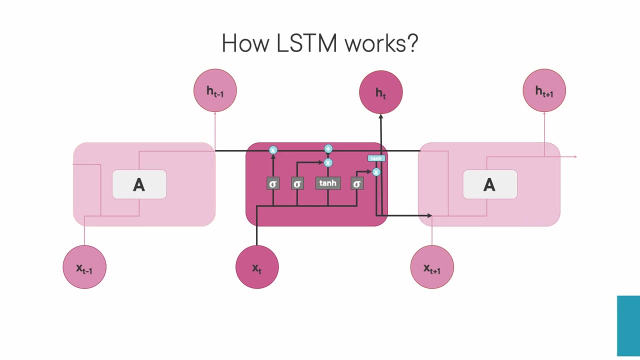 ht-1 to this central node, Then apply the tanh activation function and generate the output, which is ht. Now here's how we can present the LSTM recurrent neural network. Its repeating module has a bit different structure. Instead of having a single neural network, layer, four interacting 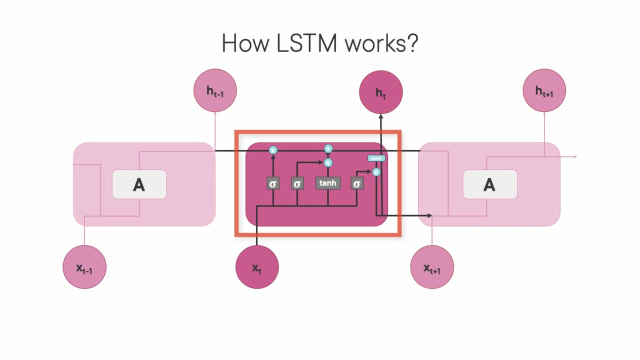 layers are communicating extraordinary. This complete box is called the LSTM cell. It has three main pods: The cell state, the hidden state and the gates Like forget, which also known as remember, input and output gate. As you can see in this diagram, it's not just a straight tanh, Of course. 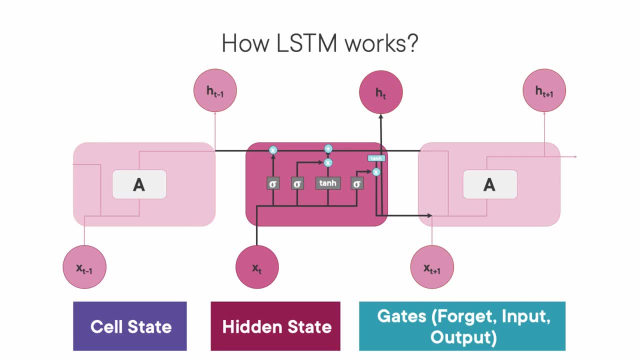 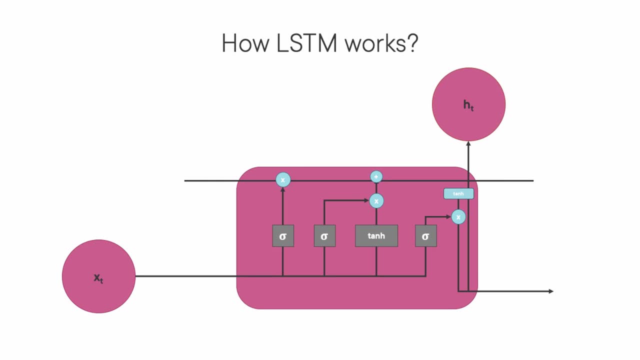 we have that component here, But in addition we have three sigmoid components, So let's expand this diagram. to get a closer look Here's first of all: just take a look at this pod in the top. We can see that the information is going in a straight line right there And we call this the 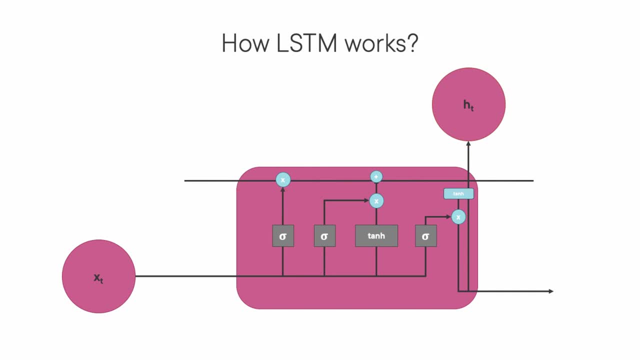 cell state, which means the state of the cell At a certain state. we are multiplying whatever this value with the state value there, So the cell state is modified. If that value is 1, then we are not modifying the state value. But why I'll explain in a few moments Next. here we are doing: 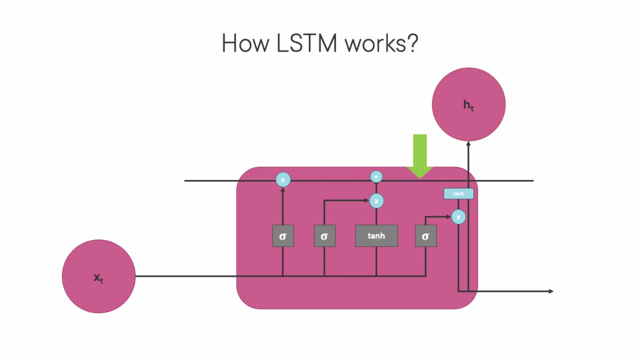 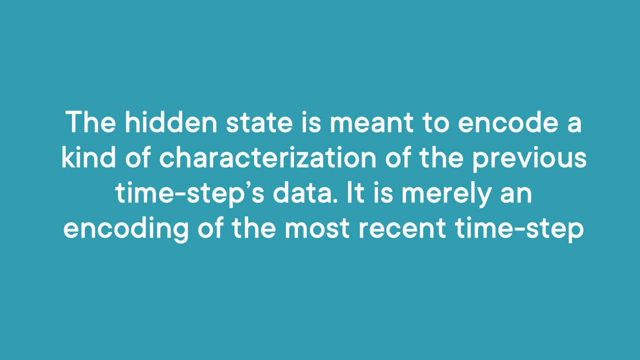 a little analysis of the cell state. We have two different types of cells. The first is the hidden state. This state is actually an encoder of the previous data, So that's the hidden state. The hidden state is meant to encode a kind of characterization of the previous timestep data. It 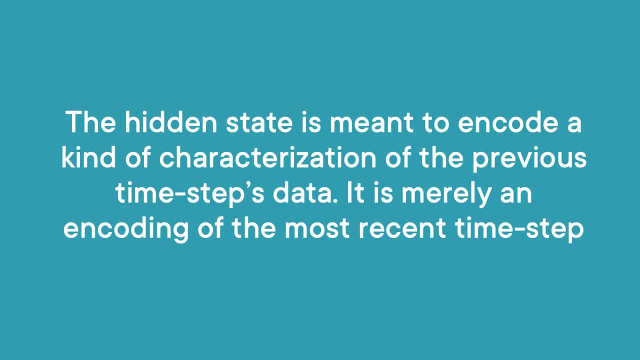 is important to note that the hidden state doesn't equal the output or the prediction. It is merely an encoding of the most recent timesteps. That said, the hidden state, at any point, can be processed to obtain more meaningful data. In other words, this cell state can be processed to create a. 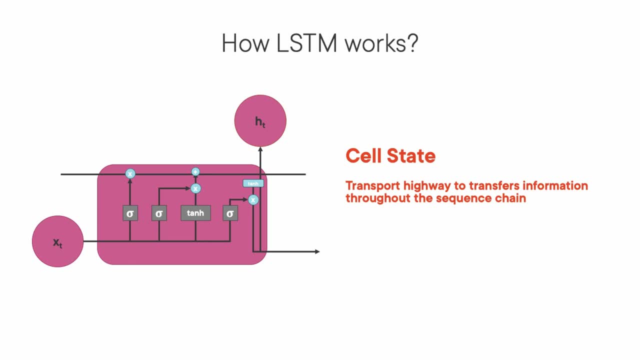 state act as a transport highway that transfers relative information all the way down the sequence chain. You can think of it as the memory of the network. The cell state can carry relevant information throughout the processing of the sequence, So even information from the earlier time steps can make its way to the later time steps, reducing the effect of short-term memory. 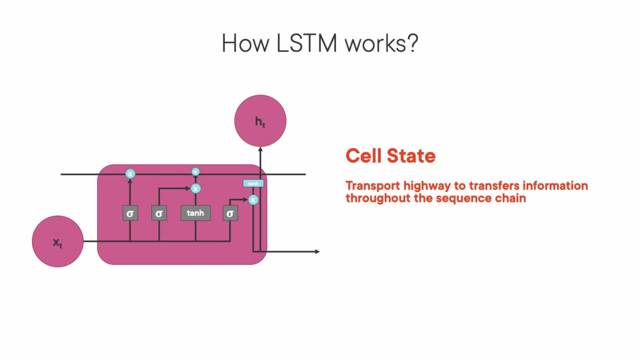 As the cell state goes on its journey, information gets added or removed to the cell state via the gates. The gates are different neural networks that decide which information is allowed on the cell state. In other words, the gates can learn what information is relevant to keep or forget. 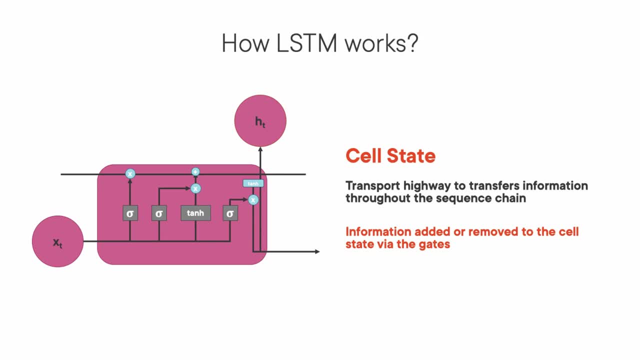 during training. We have three different gates that regulate information flow in an LSTM cell. The first one is the LSTM cell. The LSTM cell is the cell that regulates information flow in an LSTM cell. The second one is the forget gate. As you can see the highlighted portion of the diagram, This gate- 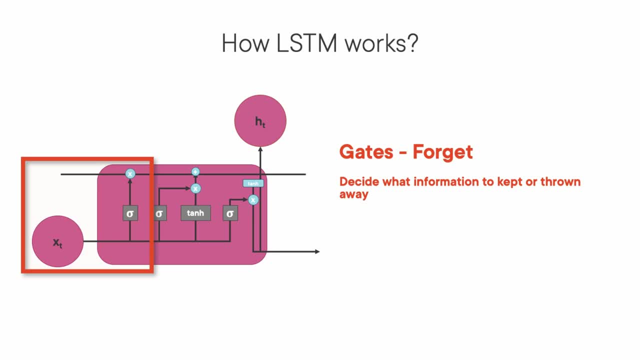 decides what information should be thrown away or kept. Information from the previous hidden state, which we called the H2-1,, and the information from the current input, which we called the XT, is passed through the sigmoid function. Values come out between 0 and 1.. The closer to 0 means. 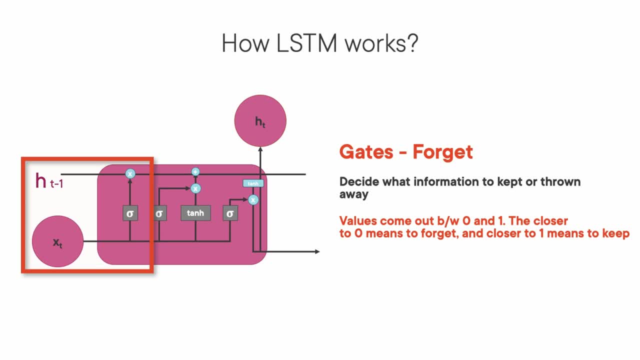 to forget, And the closer to 0 means to forget. So the information from the previous hidden state. closer to 1 means to keep, And that's the reason we are not modifying the state of the cell when this value is 1.. To update the cell state, we have the input gate In this layer. there are two. 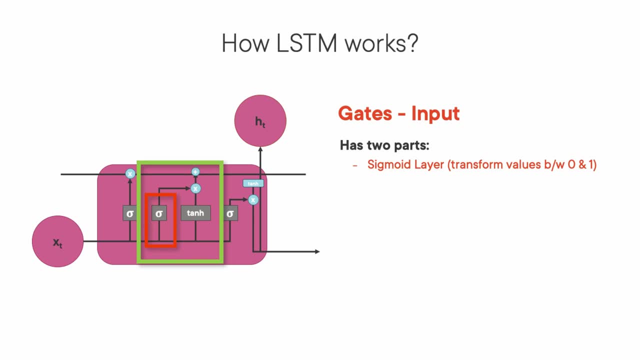 parts. One is the sigmoid function and the other one is the tanh function. In the sigmoid function it decides which value to let through by transforming the values to be between 0 and 1.. 0 means not important And 1 means important. Then the tanh function gives weightage to the values which are passed. 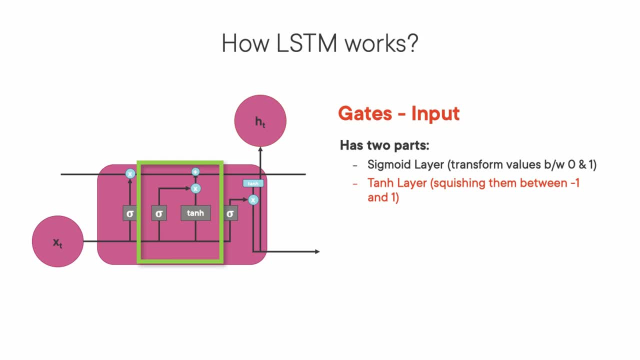 deciding their level of importance by sequencing them between minus 1 and 1.. Then we multiply the tanh output with the sigmoid output. The sigmoid output will decide which information is important to keep from the tanh output. Now, at this stage, we have enough information to calculate the cell.